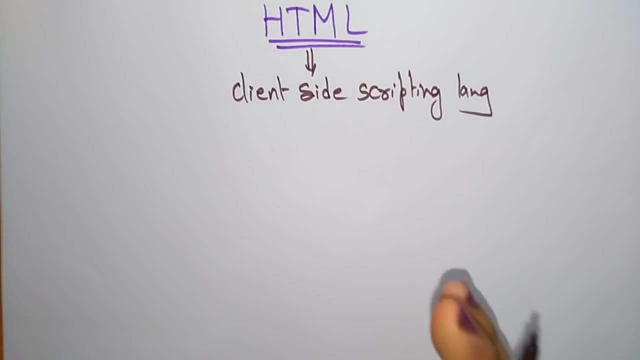 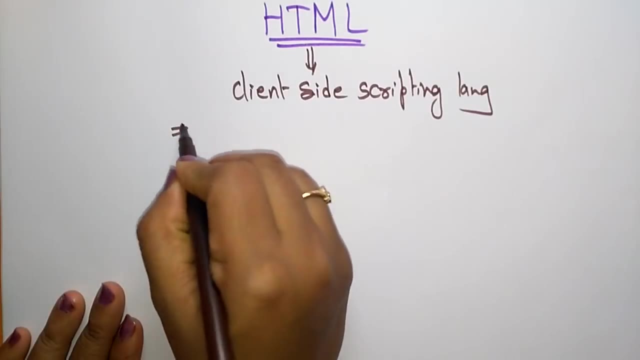 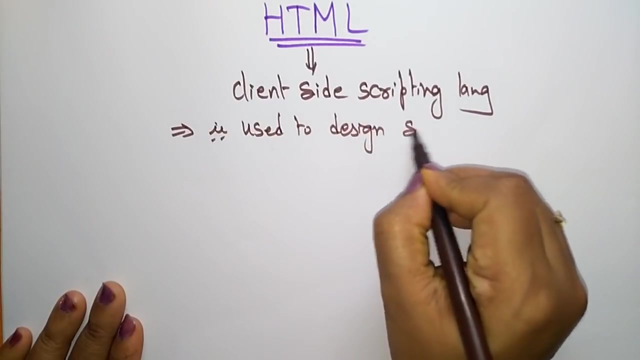 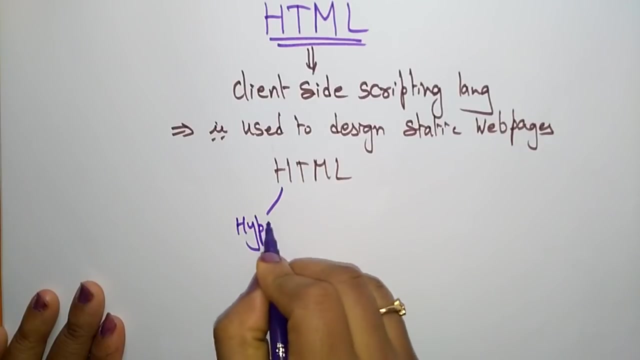 scripting language. Actually, this is used means, that is, it is used for static web pages. It is used to design static web pages. That is used to design static web pages. So what exactly this HTML was? HTML? HTML means hyper H, means hyper T means text, M means markup. 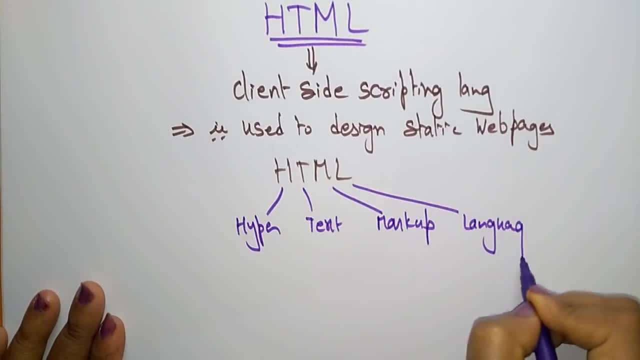 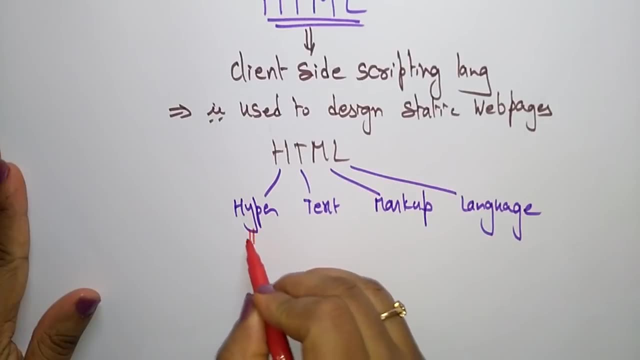 L is language. HTML means hyper text, markup language. Hyper is nothing, but it is just a link. You call it as a reference or a link. It is a link to where you have to navigate. So that is a hyper, hyper link. And next text, Text is nothing but the data or information. So, whatever the data, 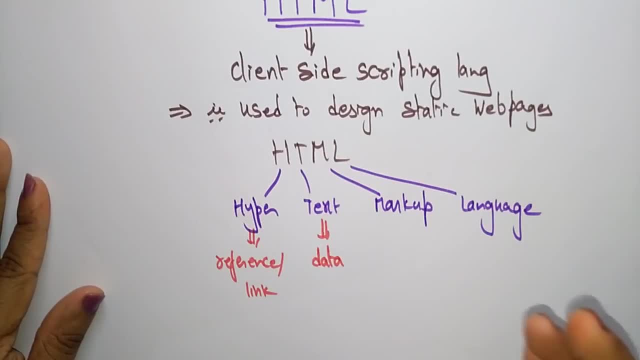 that you want to be displayed. that information will be explained in the form of text. And what about the markup? Markup is nothing, but it is a predefined terms, A predefined statement somewhat present in this HTML language. And what about the language Language is used for? 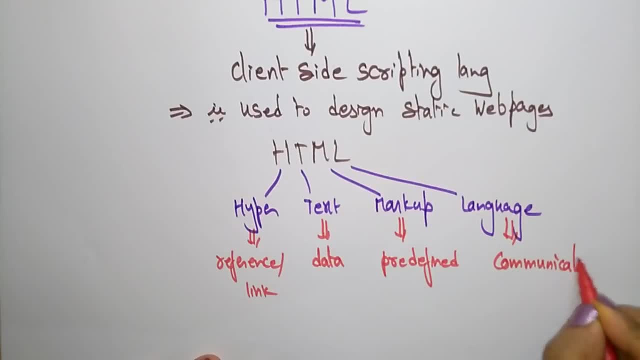 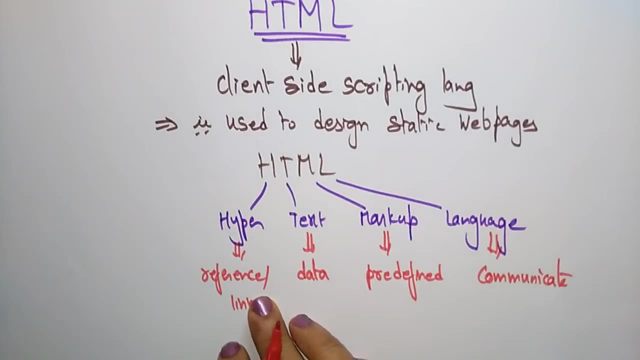 communication. So if you want to communicate, you need some language. So this is a hyper text markup language. So the thing is, whenever you are asked about what is HTML, HTML is a hypertext markup language And explain what is this. each term refers to Hyper means, reference, link Text. 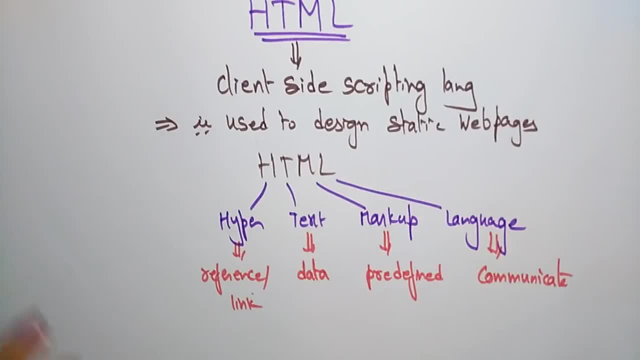 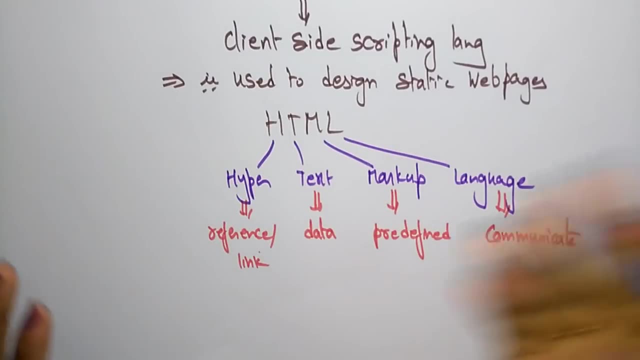 is nothing but a data Markup, is a predefined And wherever the language is nothing but complication. So HTML is not a programming language. So I already said, it is not a programming language, Just like Java See. so like that it is not a programming language, Just it is a markup. 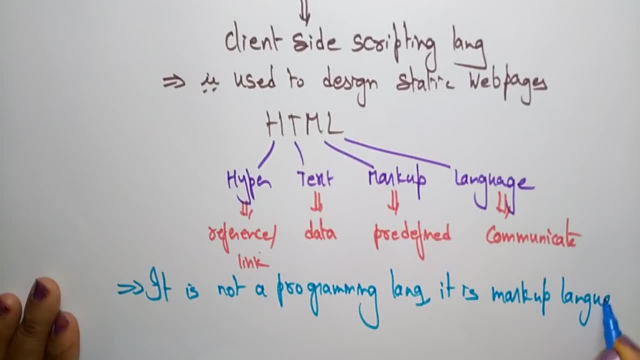 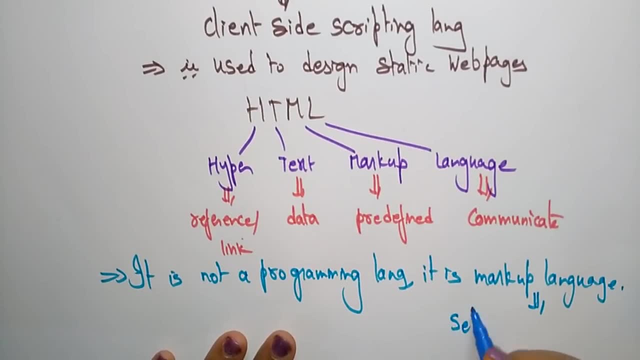 language And it may be called as markup language. The markup language is a set of markup tags. So in this markup language we are having set of markup tags. That means this markup language consisting of the syntax, that consisting of everything in the form of tags, Set of tags. 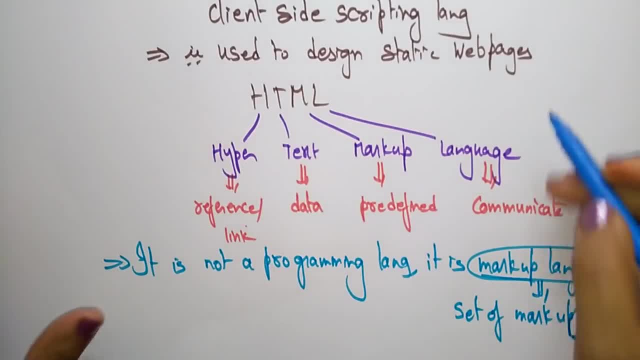 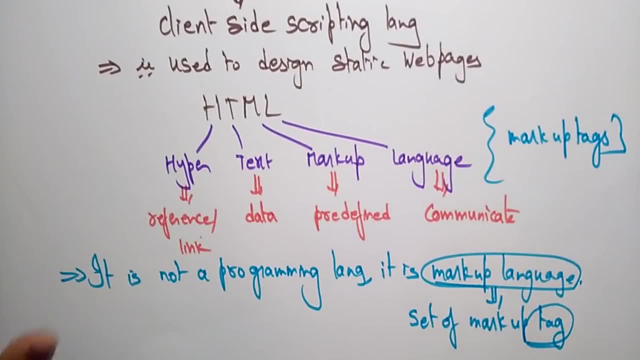 will be present. So this hypertext markup language consist of markup tags. So in this hypertext language, that complete language is in the form of tags, the markup tax or use it to describe the web pages. so these markup tags use it to describe web pages. okay, so don't be confused. HTML is: is: 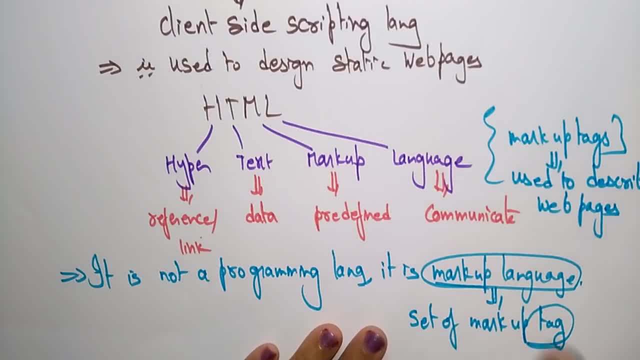 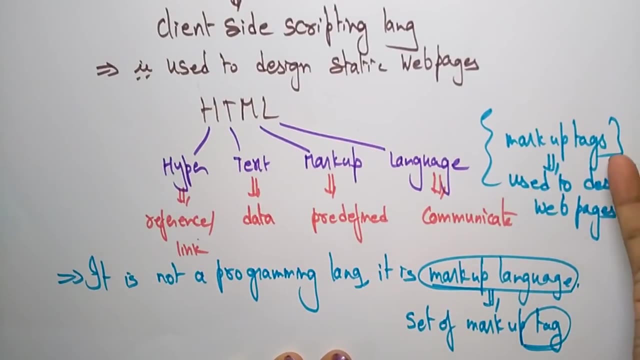 not a programming language. you just call it as a markup language. what exactly that markup language consists of? whereas programming language is in the form of English, like sentence, whereas markup language is just a set of markup tags. it is in the form of markup tags. so what that markup tax? 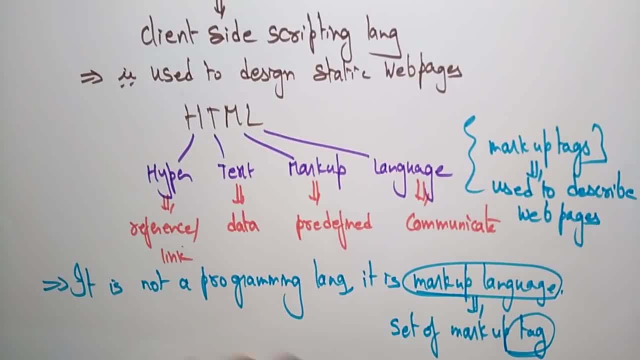 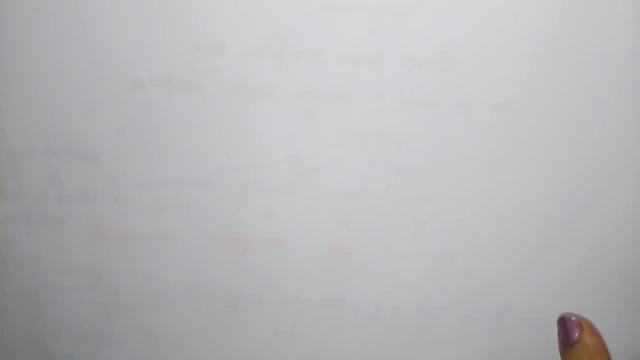 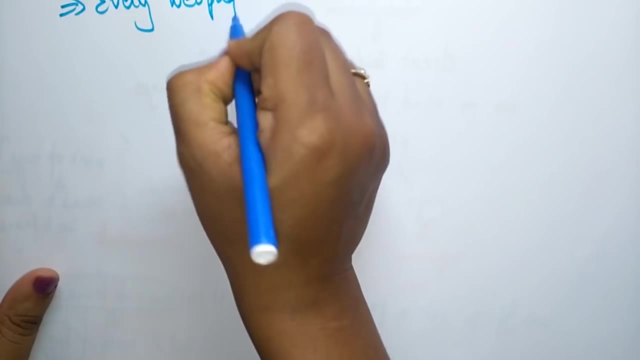 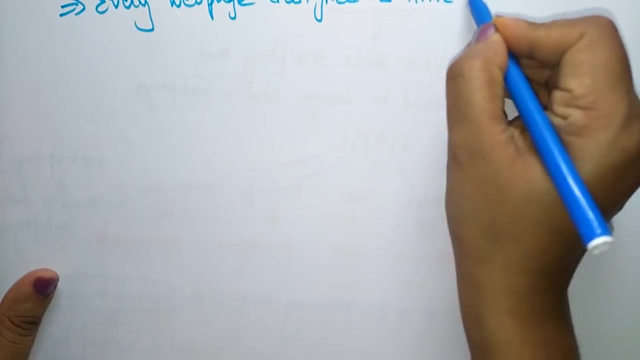 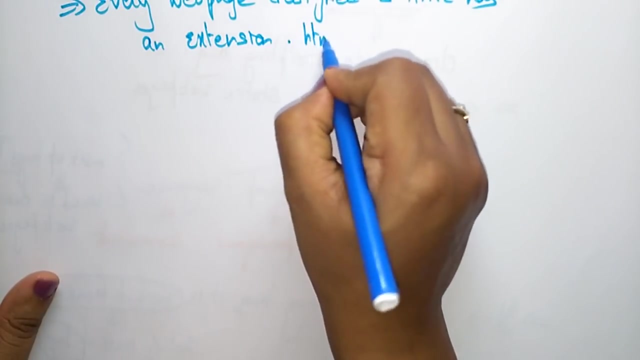 consists of. it is that markup tax is used to describe the web pages. so here, whatever the web page that you want to design, that every web page is designed in H is. let me write that every web page is designed as HTML has an extension. it was saved in the form of extension like dot html or dot htm, so 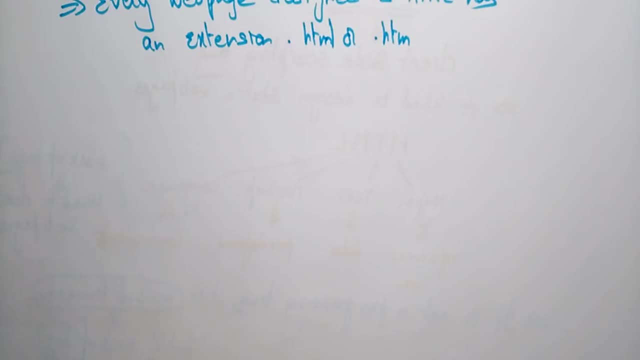 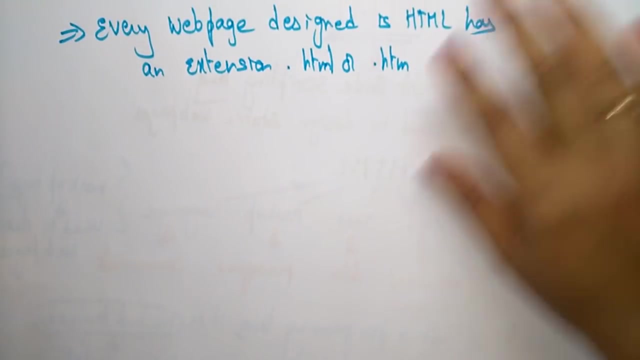 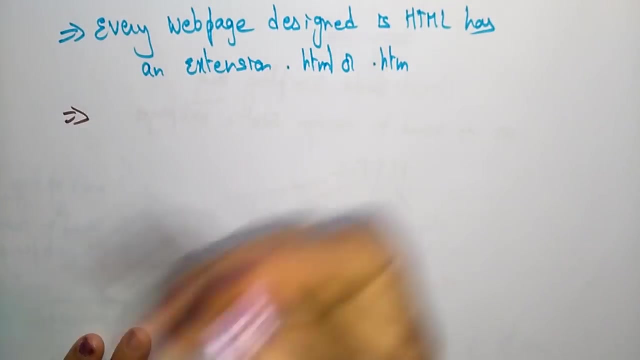 whatever the program you are writing that is in the form of tags that should be saved by using the extension dot html or dot htm. okay, where you write this HTML programs, so we will the editor. we use it to design this HTML static web pages, or you can use notepad or notepad plus plus. so either you use these editor or notepad plus plus. 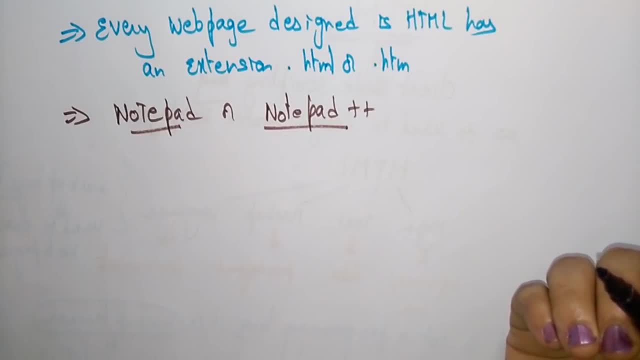 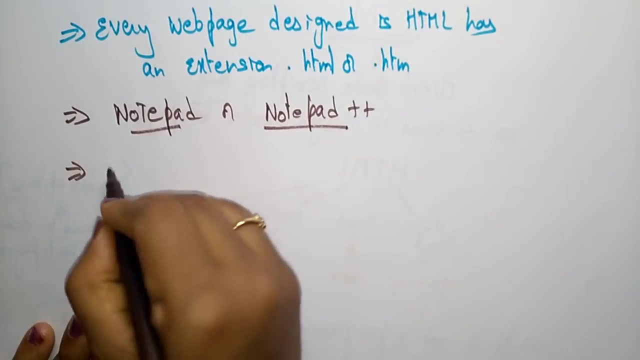 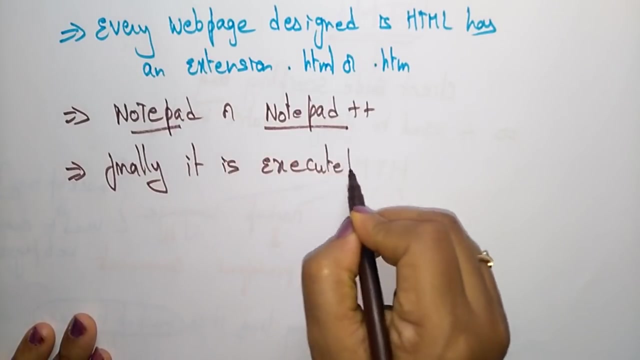 editor to write the HTML language and here this: whenever you have written that, you just save it, as here, every HTML script will be executed in any web browser. so, finally, it will be executed on. it is executed in any web browser. okay, so this hypertext markup language: whenever you have saved that, it. 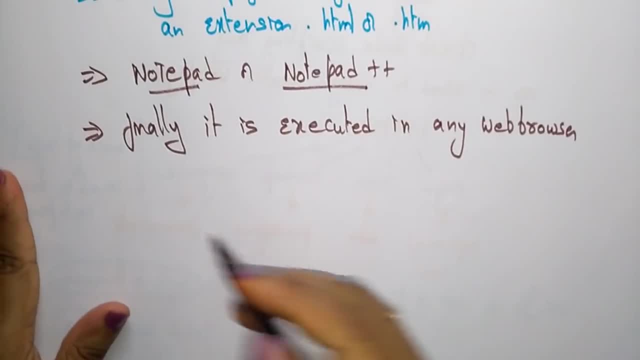 will be executed in any web browser. so let me write a simple syntax above of this script here. wait it: html. i said that html is a markup language. it is not a programming language, the markup language consisting of markup tags. so this is the tags representation: doc type: html. 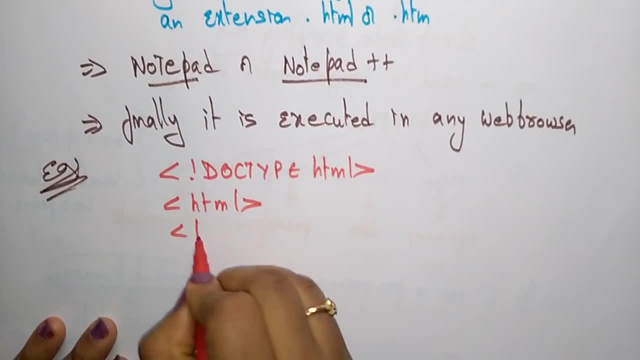 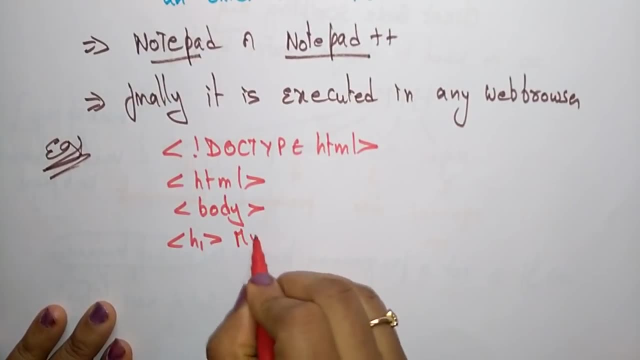 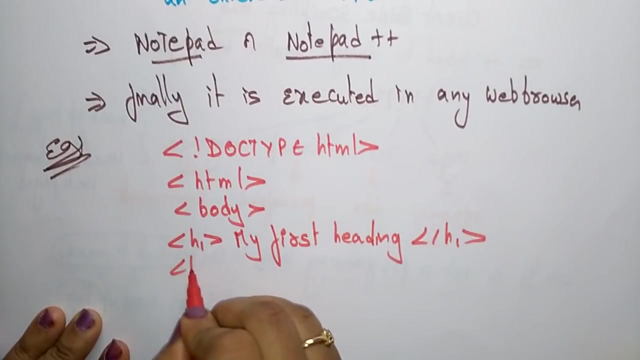 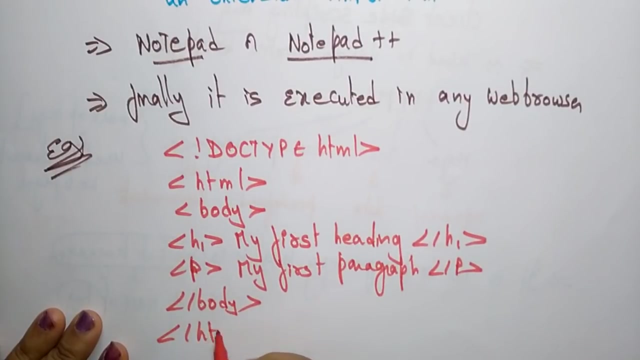 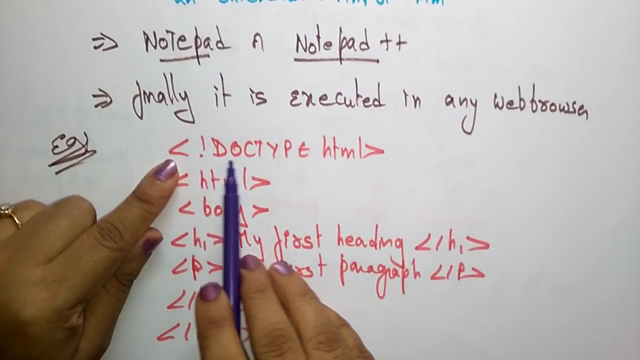 first let me write the program, after that i'll explain what exactly these tags are. my first heading, and then this is one of the tag paragraph. my first paragraph: close the body, close html. so this is a markup language, so what this tags represents. so here the doc type html is a marker language. 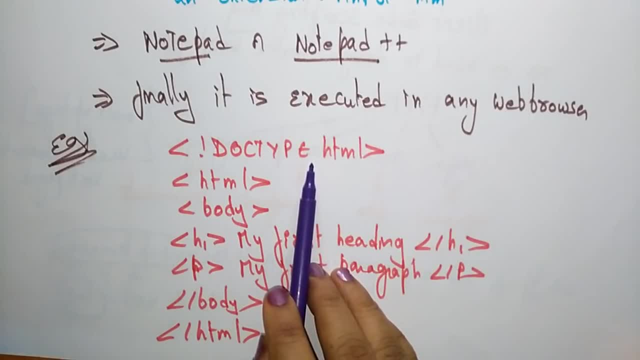 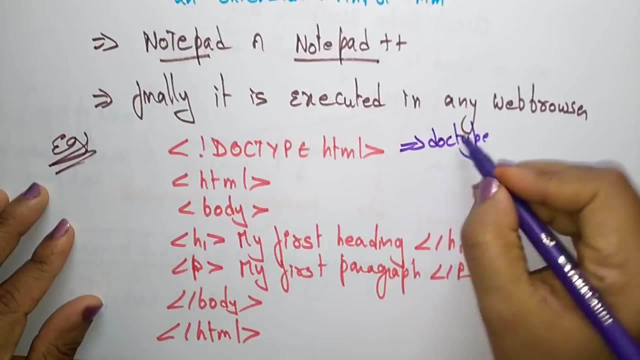 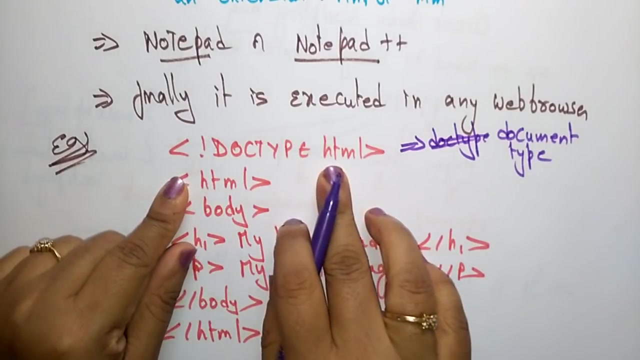 so this is a marker language. so what this tags represents is nothing but declaration of it's- just declaration defining the doc. document type. it's nothing but whatever the text you are writing is document, document type of text we are writing. so that is a representation here and whatever the statements that you are writing, that should be. 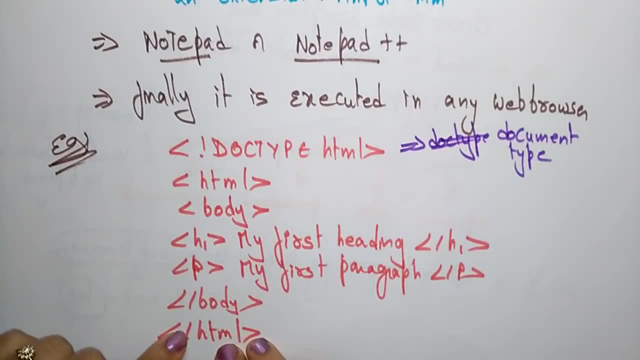 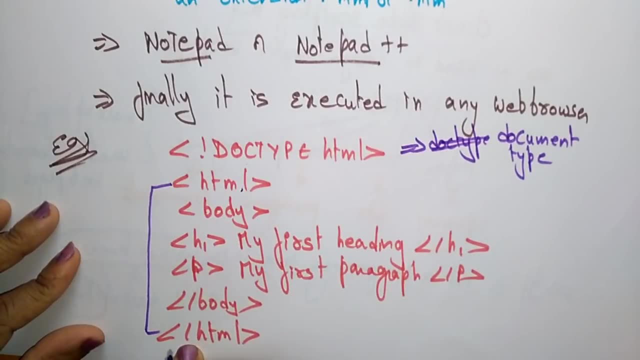 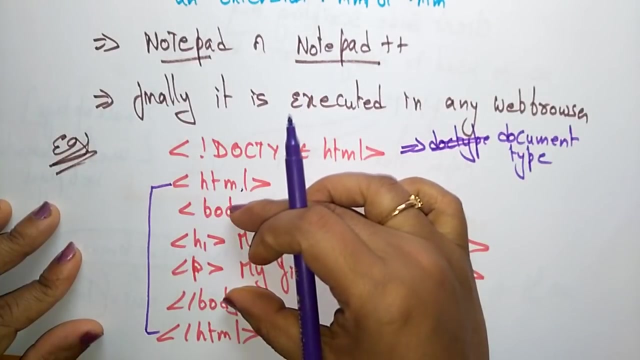 started with the open tag and this should be the close tag. so this is the html, this is the starting html and of the statements. you have to close by using the backslash. okay, so this is a text between whatever the text between the html describes the web page. so in between this html, open and the 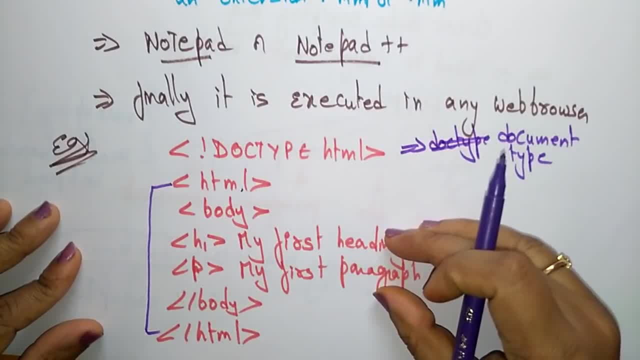 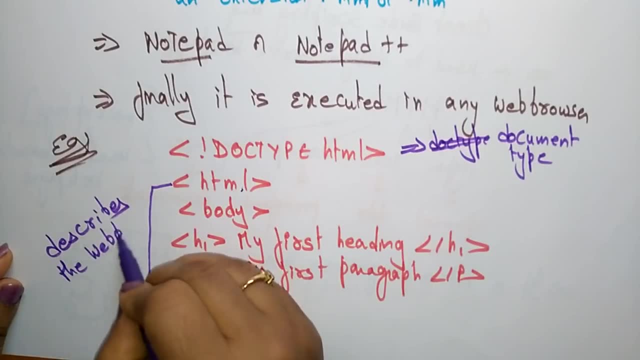 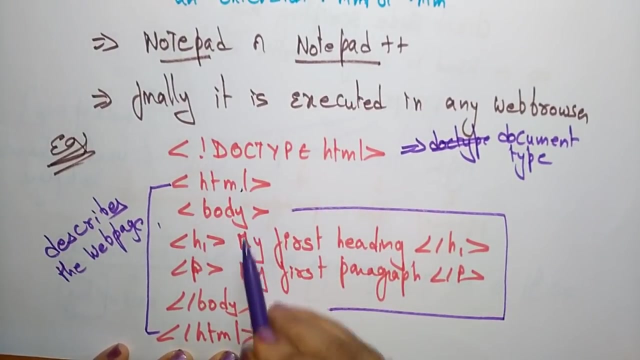 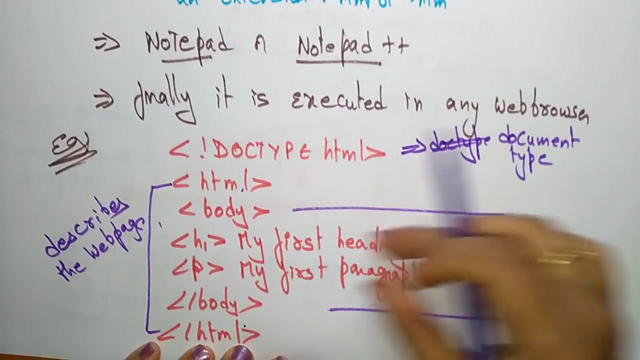 close. whatever the text that is present in between the stacks describes web page, describes the web page. then what about this body? so here, whatever the body that is consisting of open, starting tag and ending tag of the body, so this body here, the text between the body. whatever the text that is present between the body is a visible page content.